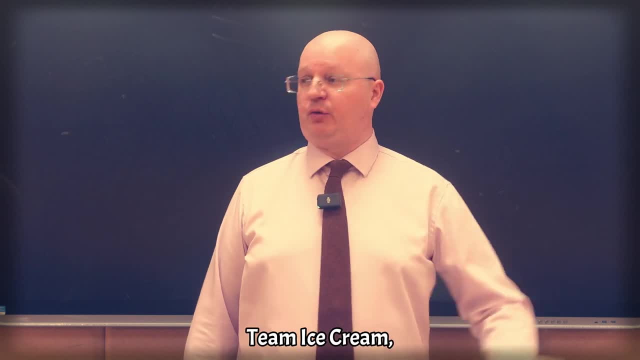 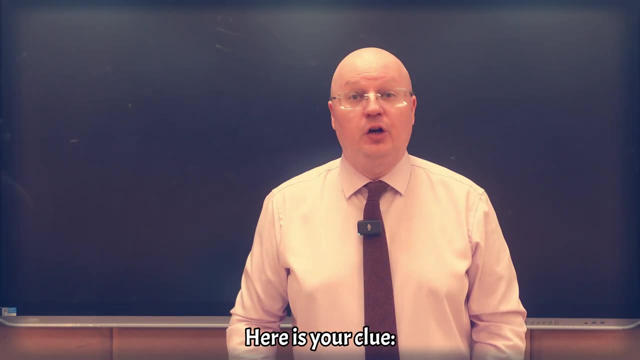 Team. do you want to go? Do you want to go? Good, I picked 3.. 3 it is. Here's your clue. It's something your teacher gives you to do at home after school. Hurry up and get it. 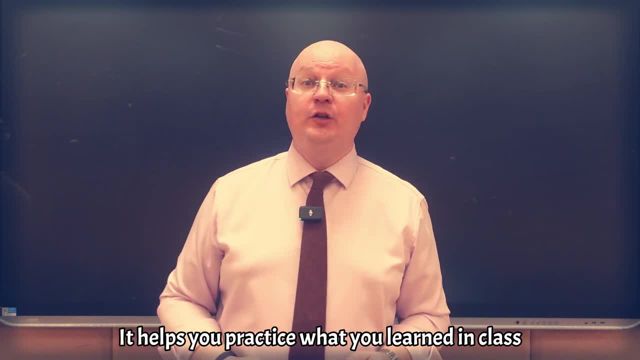 And you can do it right away. Huh, Fine, take my hand. Okay, I got it. Take me the chair for you. Case closed- Telesares, It helps you practice what you learned in class and get better at it. 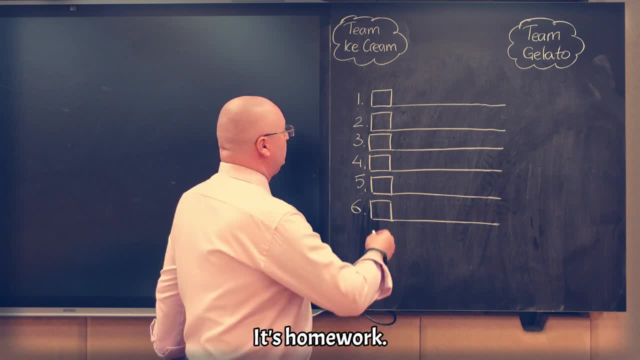 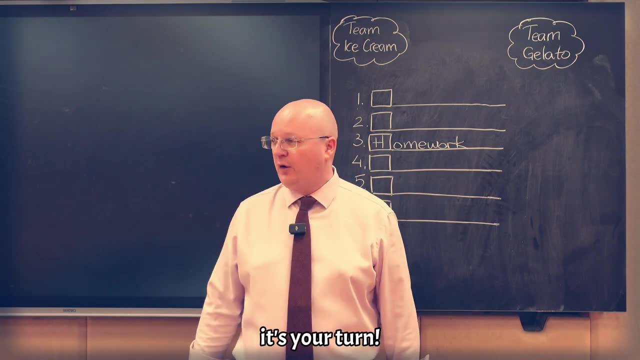 Homework, Homework. Yes, Yes, that's right, It's homework. Very good, Here we go Homework. Good job, Team Gelato. it's your turn. Which number do you pick? I pick one Smart choice. Here is your clue. 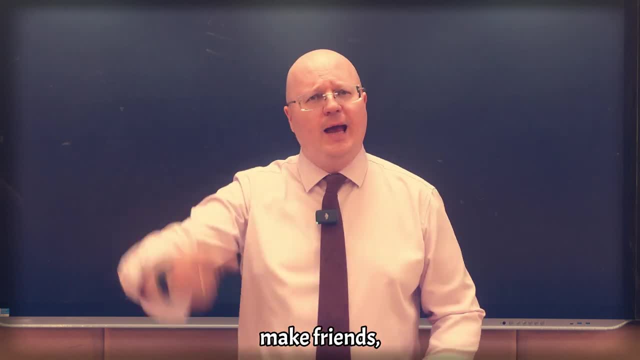 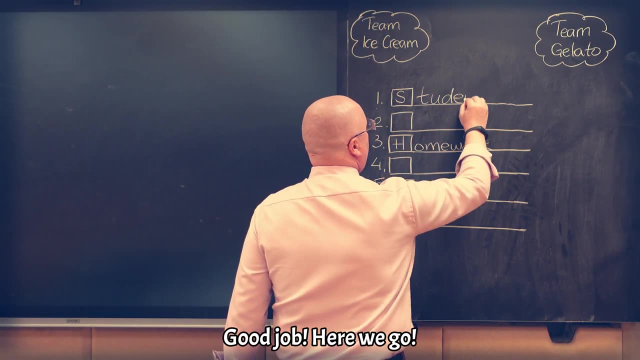 This person goes to school to study, make friends and get smarter. Student- Yes, that's right, It's a student. Good job, Here we go. Good guess. Are you ready to guess the mystery word? No, Not yet. 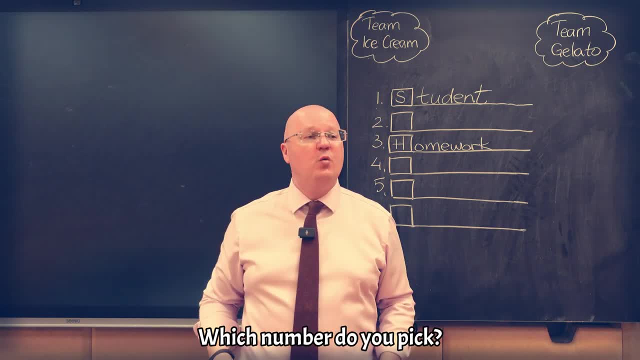 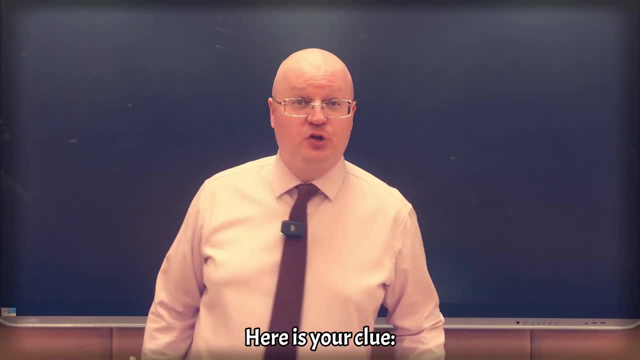 That's okay. That's okay. Team Ice Cream. Team Ice Cream. it's your turn. Which number do you pick? Number six, Number six, Number six. you say Okay, Here is your clue. It is a small computer that you can carry with you like a book. 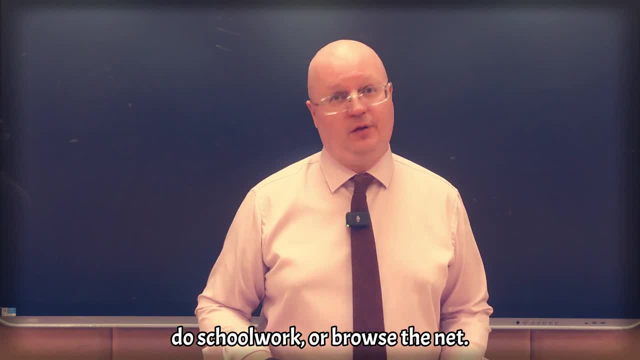 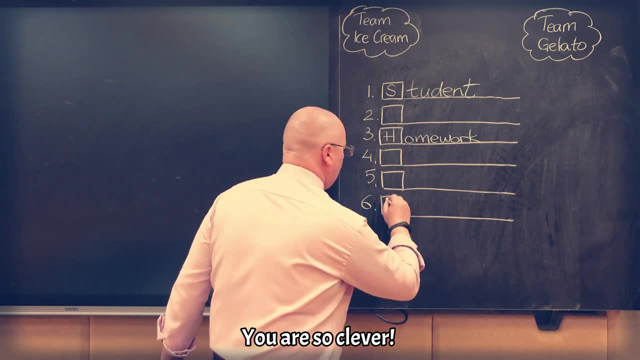 You can use it to play games, do schoolwork or browse the net. Laptop, Laptop, Yes, that's right, it is a laptop. You are so clever, Oh my God, Laptop So clever. Are you ready to guess the mystery word? 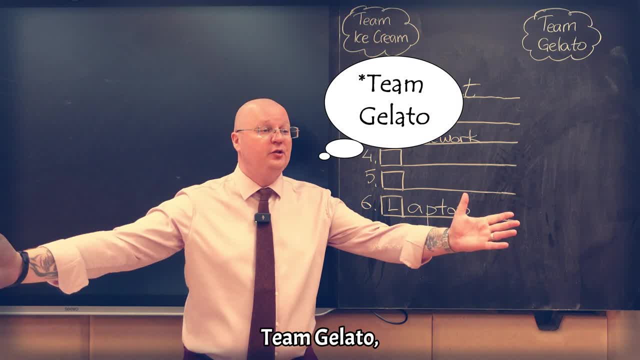 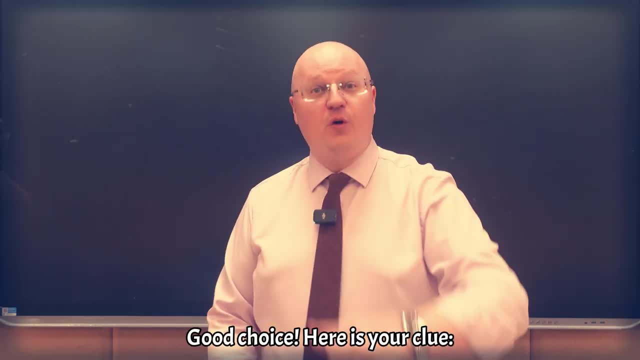 No, not yet. That's okay. That's okay, No problem at all. Team Ice Cream. it's your turn. Which number do you pick? Number four, Good choice. Here is your clue. It's like a school class, but you don't go to a classroom. 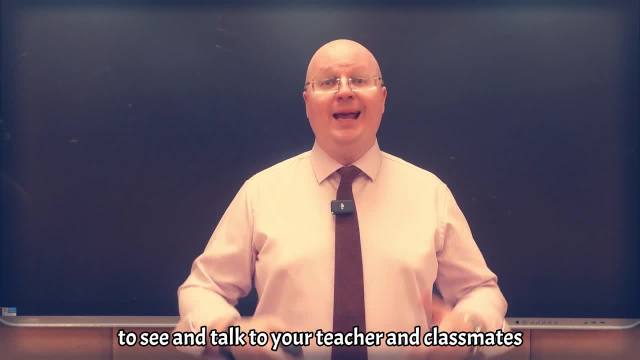 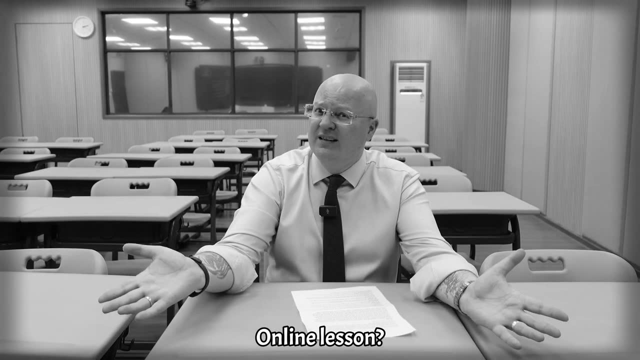 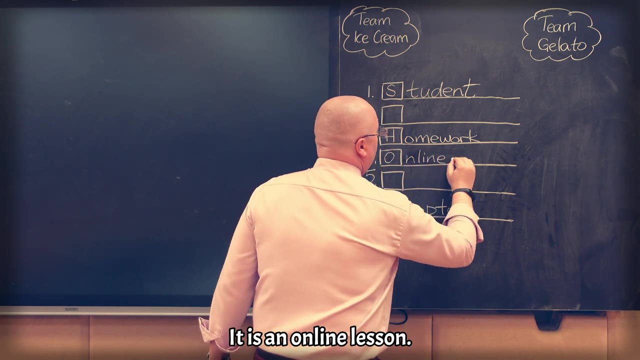 Instead, you use a computer to see and learn, And you can see and talk to your teacher and classmates on the screen. The answer is two words: Online lesson, Online class. Yes, yes, that is correct, It is an online lesson. 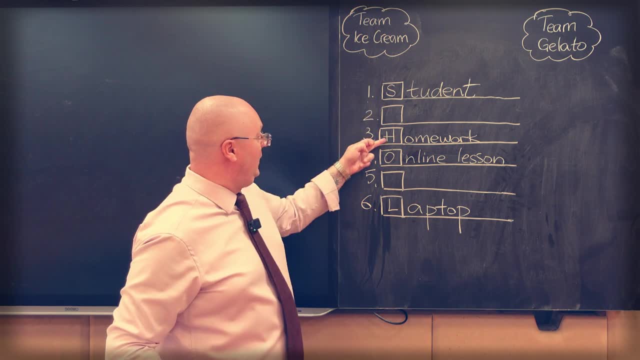 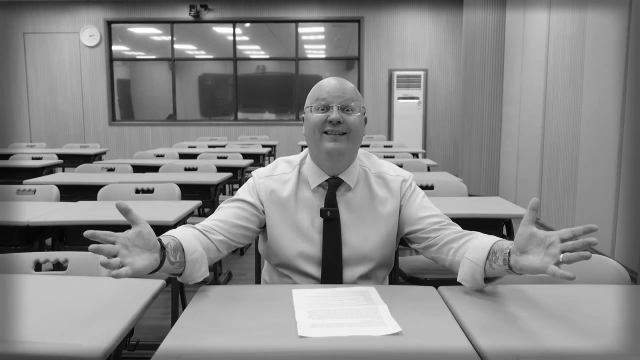 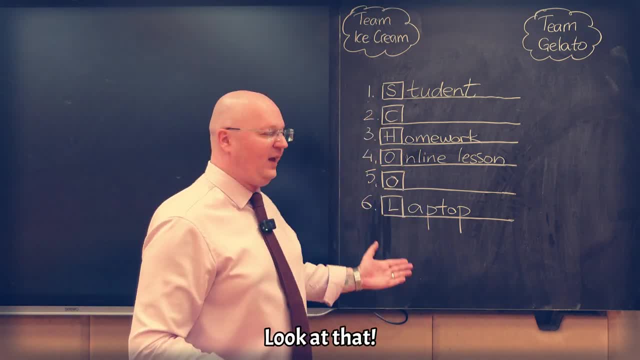 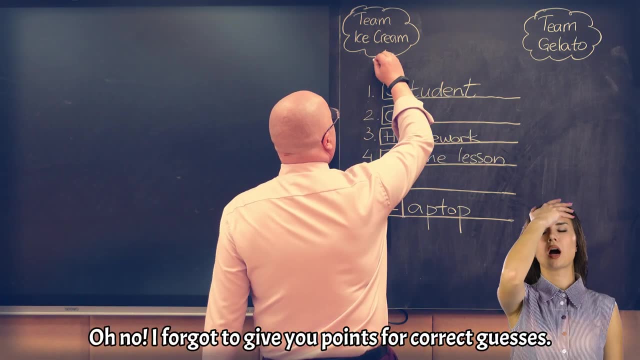 That is correct, Excellent School. Look at that. Good job. Team Gelato, You get five points. And oh no, I forgot to give you points for correct guesses. Team Ice Cream has two points. Team Gelato has two points. 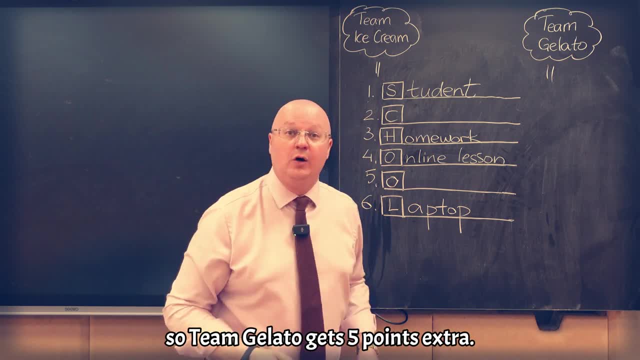 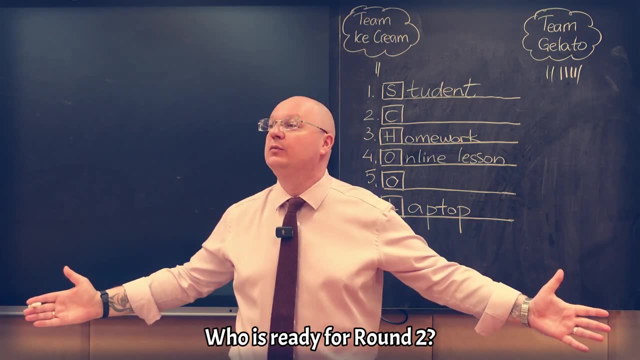 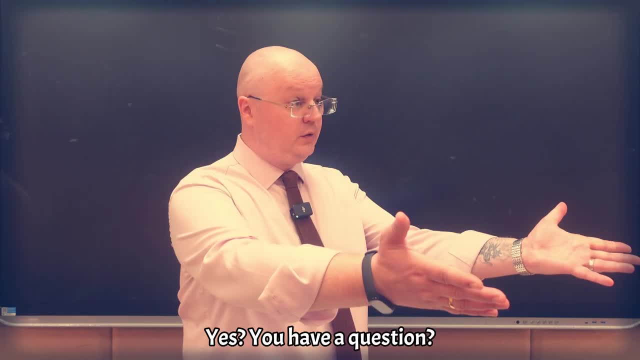 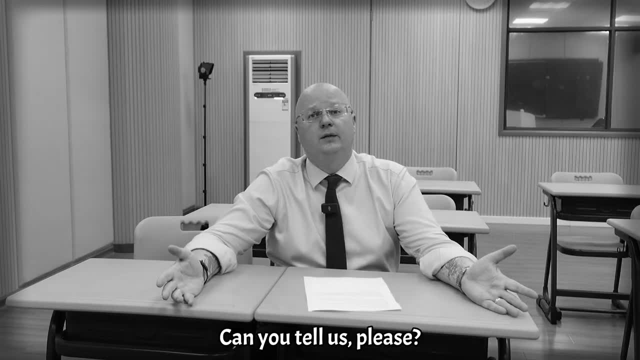 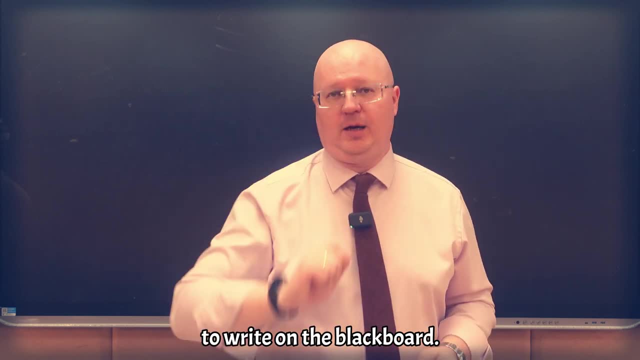 What is it? Teacher, teacher, teacher? What are words number two and five? Can you tell us, please? I like your curiosity, my dear. Number two is a special stick that teachers use to write on the blackboard. It's usually white. 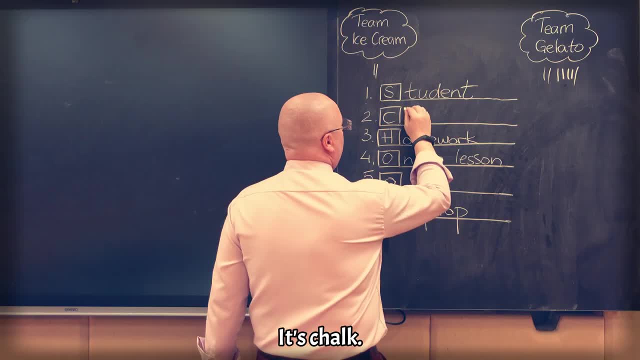 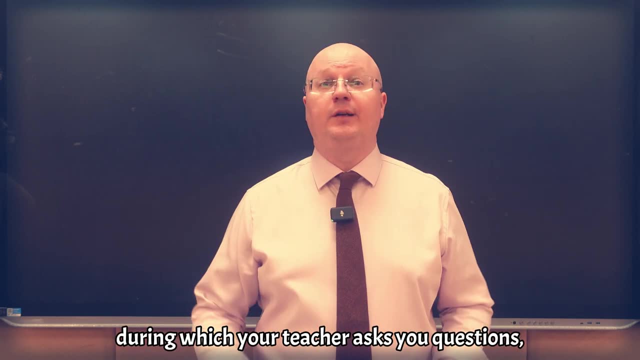 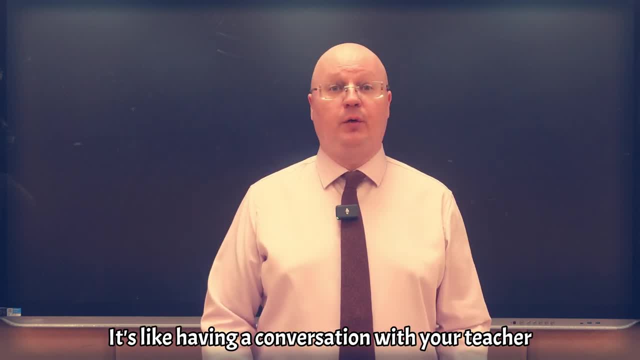 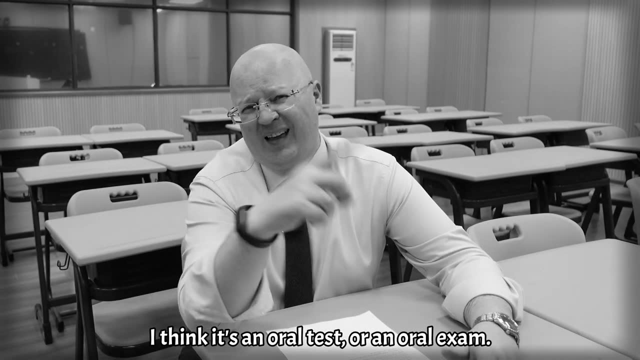 It's like. it's like having a conversation with your teacher to show what you know. The answer is two words. I think it's an oral test or an oral exam, One of those things. Yes, yes, yes, it's one of those things. 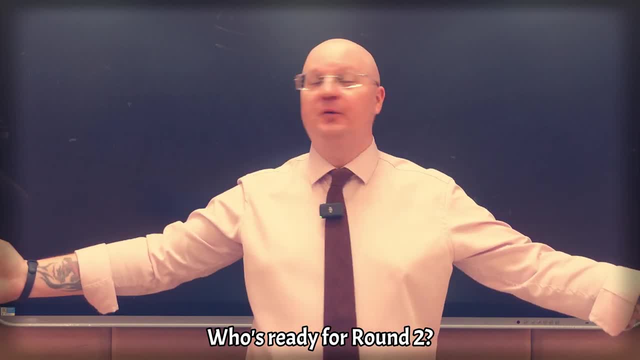 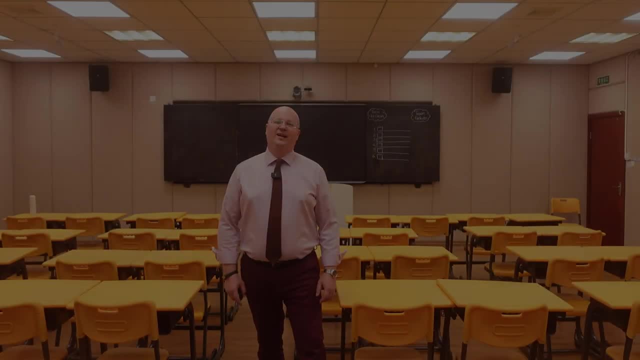 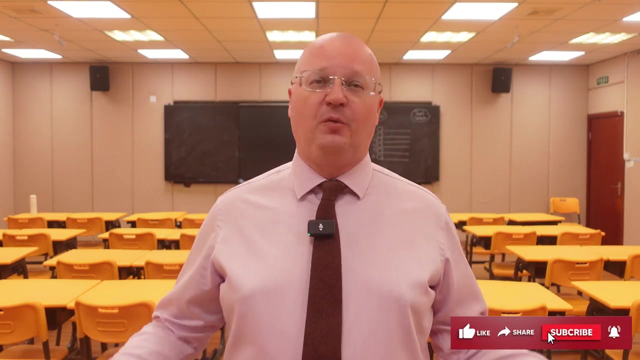 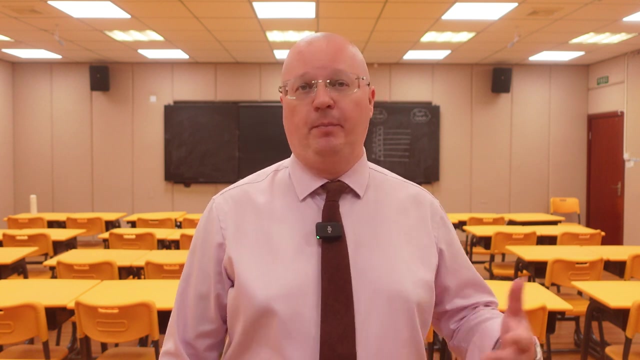 Yes, you're right. Well done, well done. Who's ready for round two? Anyone? Well, I hope you enjoyed this video And, if you did, please like and subscribe for more educational content. If you'd like to support my channel, please consider becoming my patron or. 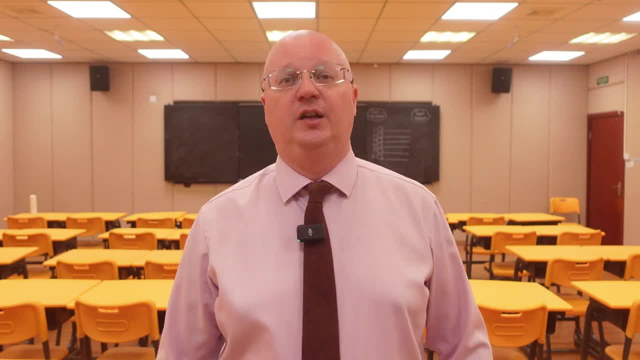 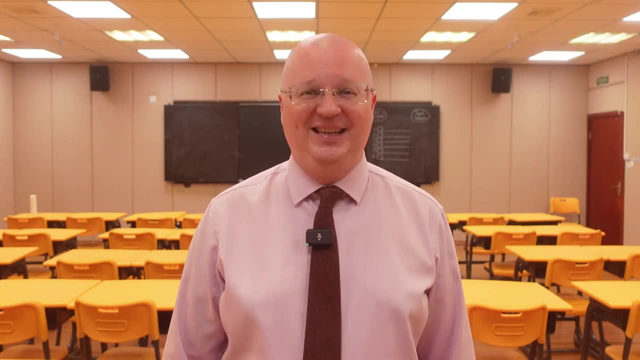 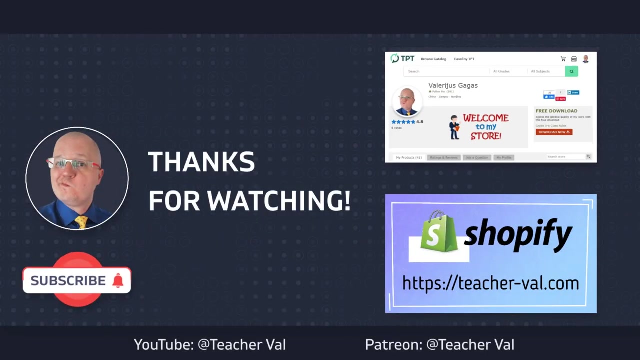 channel member or leave a small donation by clicking on a super thanks icon, The one with the dollar sign inside. Many thanks and happy teaching. Bye, Bye.